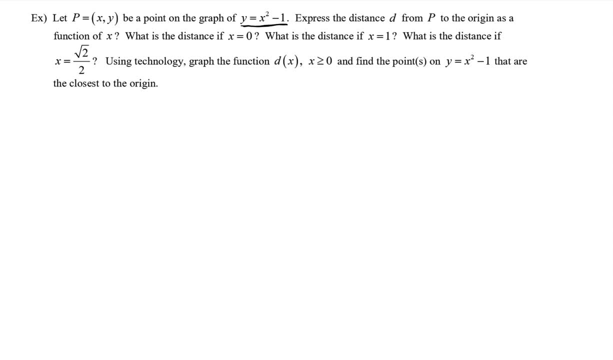 Any point on this graph, right here, the graph of this parabola. Notice, it is just the squaring function shifted down one. And what if I want the distance between that point and the origin on the coordinate plane? Can we come up with a function that models that distance? 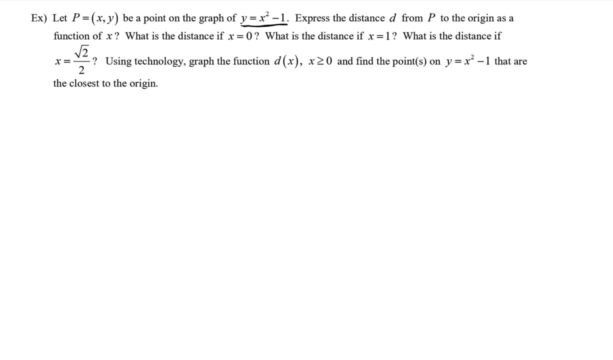 Well, let's see if we can. I like pictures, I like to know what things look like visually. So this is just the squaring function. It's been shifted down one, So let's go ahead and draw that real quick. So here's our coordinate plane. 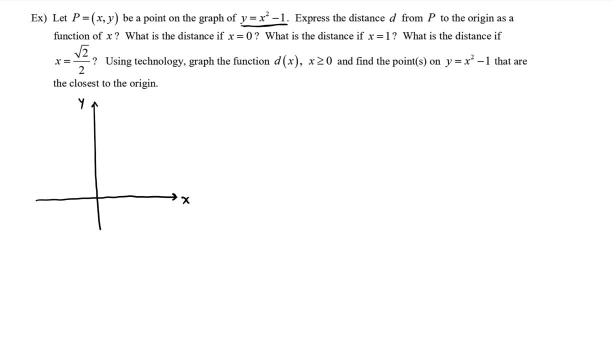 The squaring function usually has a vertex at 0, 0, but it's been shifted down one, So it'll be down here. If you plug in 1, you get 0.. If you plug in negative 1, you get 0. 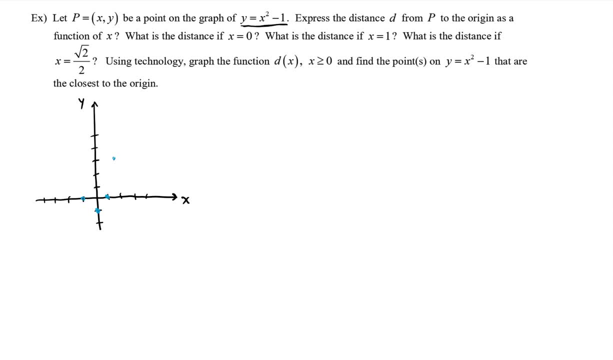 If you plug in 2, I think we're going to get 3.. And then negative 2 will give us 3.. So it's going to be the squaring function's graph, this parabola shifted down one. Now we're letting P be any point on that parabola. 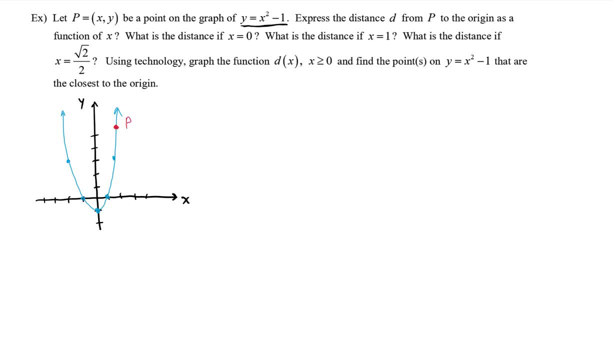 So, for example, if this was the point P, well that point would be x, And then to get the y-coordinate, it's just x squared minus 1. And then from that point to the origin, that's a distance. 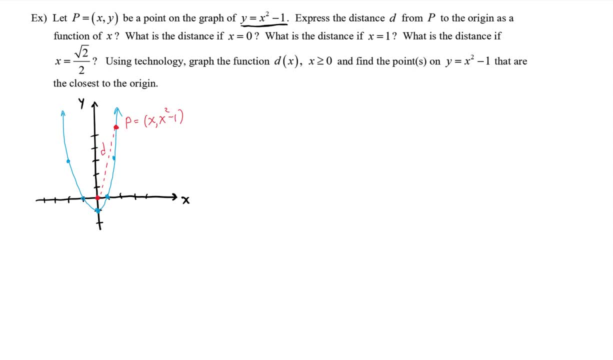 Some unknown distance. But notice, if I picked, say, this point P, I would be even closer to the origin. So, depending on what the point is, I am closer to the origin or further away from the origin. So we're trying to find what point specifically is closest to the origin. 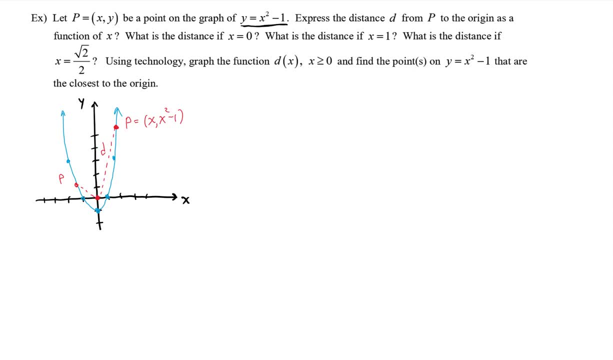 And from the picture it looks like there's going to be two points that are the closest It could be two points. We have some symmetry going on here, So let's see. Well, We know the distance formula. We derived that earlier. 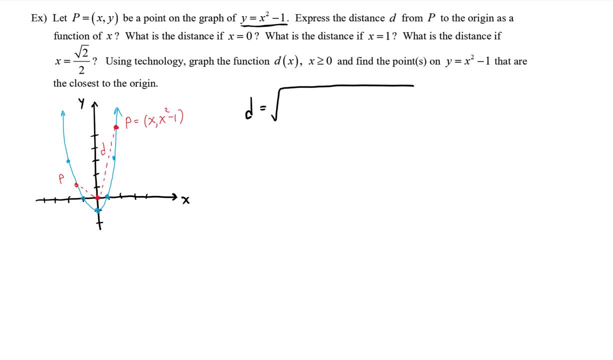 So to get the distance between any two points, it's the principal square root of what. Well, you subtract the x-coordinates and square it, And then you subtract the y-coordinates square and add them together, Do the principal square root of that and you get the distance between those two points. 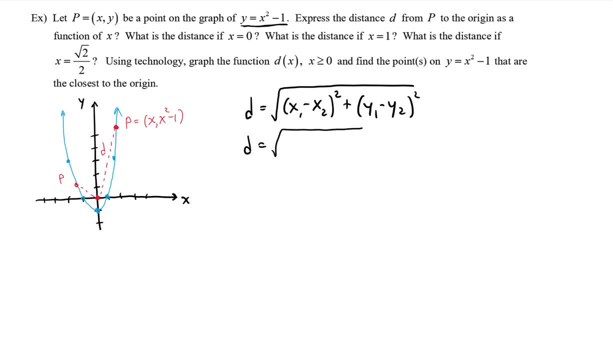 So if I want to do the distance between this point here and the origin, it would be x minus 0. And this point in the origin, the y-coordinates would be x squared minus 1 minus 0. So if we collect like terms, start to multiply this out, we would get x squared x to the fourth minus 2x squared plus 1.. 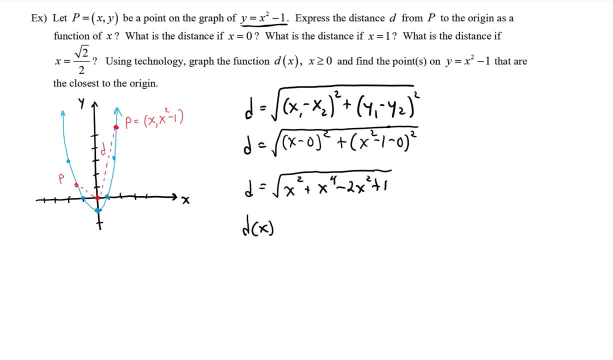 And now we can collect like terms. The distance, depending on what the x-coordinate is, is going to be x to the fourth, Minus x squared plus 1.. So now I have a function. So right, here's a function. I'm going to go ahead and highlight this bad boy. 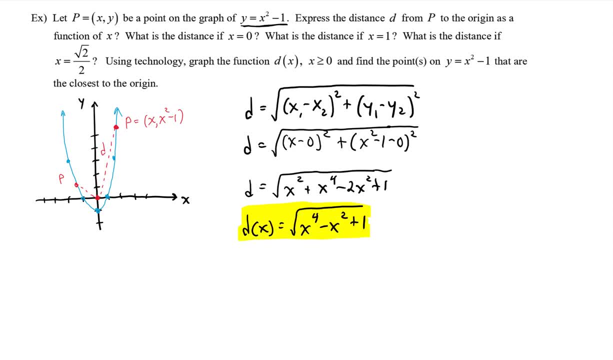 I have a function where if I plug in an x-coordinate, it gives me the distance between that point, that location, on this relation, this function, this parabola, and the origin. So now I can just keep plugging in x-coordinates and keep getting different distances and see, you know what the shortest distance is. 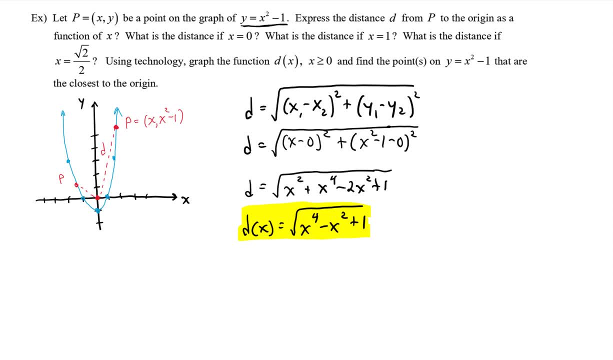 To get an idea of what the closest point is. Now, we're not going to sit and plug in a whole bunch of x-values. It turns out there's a quicker way, But let's play around with a few. So what if x was 0?? 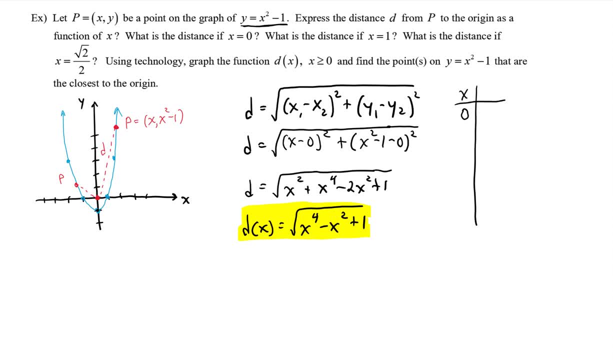 What if we did this point down here? Well, I think we'd agree. that's one unit away by looking at the picture. So let's see: 0 to the fourth is 0.. Minus 0, squared is 0.. Plus 1 is 1.. 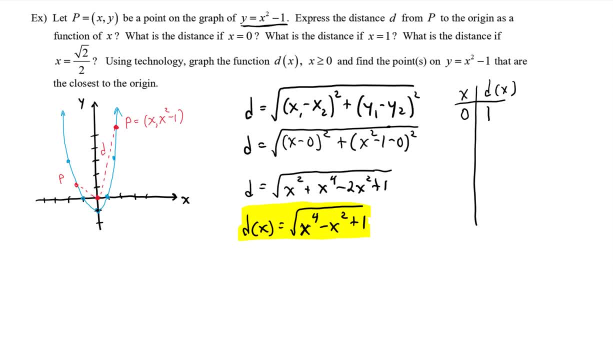 And the principal squared of 1 is 1.. So that's That distance is one unit. So if I pick the x-coordinate 0, the vertex, it's one unit away from the origin. But we knew that from our transformations and our knowledge of this function. 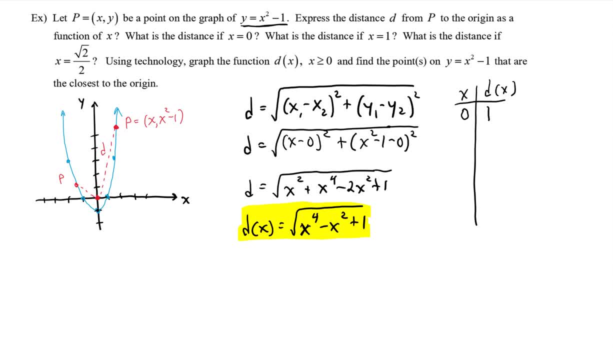 What if the? What's the distance going to be if x is 1?? So what if I'm here or here? So if x is 1,, 1 to the fourth is 1.. Minus 1 squared is 0.. 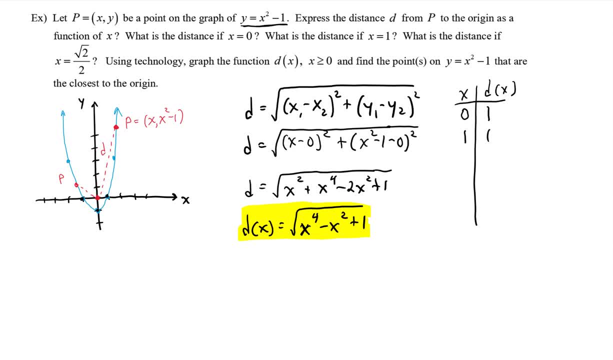 Plus 1 is 1.. We're back to just a distance of 1 again, So- And the same would be true if I was over here- at negative 1.. So we just found three locations that are all one unit away from the origin. 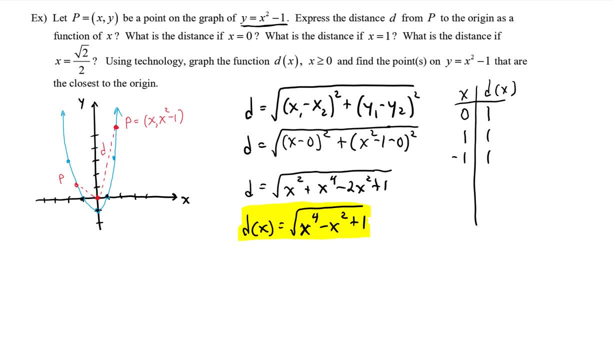 The question is: is that the shortest distance, Or is there a point that's even closer? Is there a point that's even closer? Well, rather than just plug in and guess and check, I've got another one for us to try here. 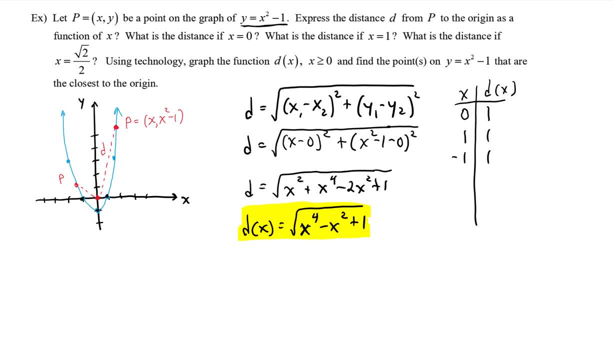 Square root of 2 over 2.. And then we're going to use some technology, So if we plug in square root of 2 over 2. Let's see what we get, So that one's a little bit trickier for the arithmetic. 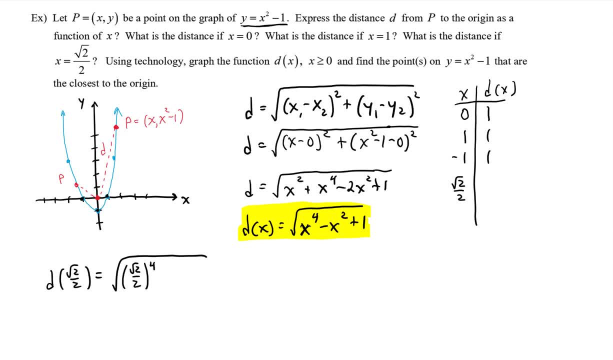 So we do square root of 2 over 2 to the fourth, Square root of 2 over 2 squared plus 1.. Let's see That would be 4 over 16 is 1 fourth, And then that would be 2 fourths, which is 1 half. 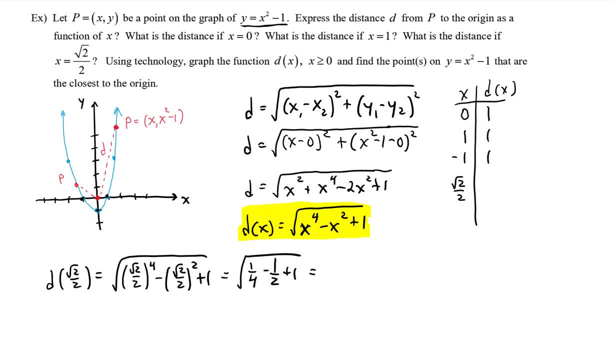 Plus 1.. So that would be- let's see negative- 1 fourth would be 3 fourths. So we'd get principal square root of 3 over 2.. The principal square root of 3 is about 1.7.. 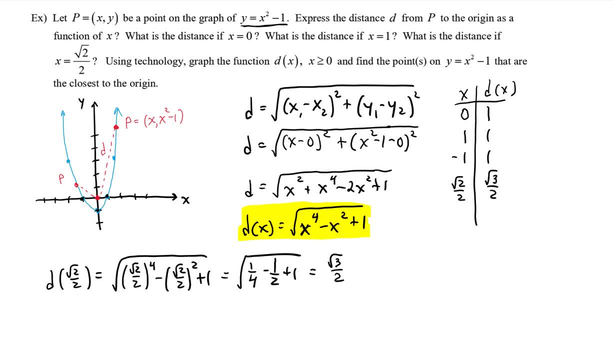 If you cut that in half you get about 0.85.. Now, of course that's without a calculator, So that's just some very rough estimating there. But notice that distance is shorter than 1.. So we did find an x-coordinate whose distance is: 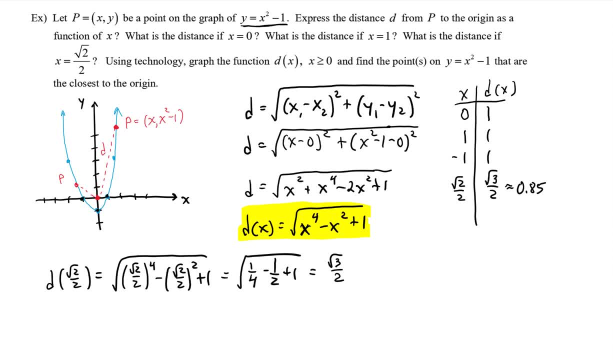 less than 1 from the origin. So, again, though, the question is: is that the x-coordinate that gets you a point closest to the origin on this parabola? Well, let's use some technology to find out. Let's speed this up. 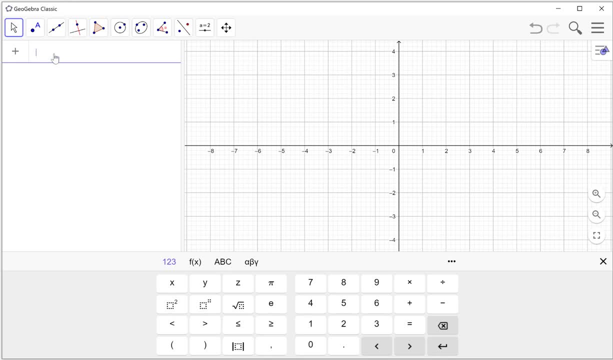 Okay, so we're going to go ahead and use GeoGebra here. Let's graph our function. Go ahead and call it d, And it's the square root of x to the 4th minus x, squared plus 1.. So that is the function that models the distance. 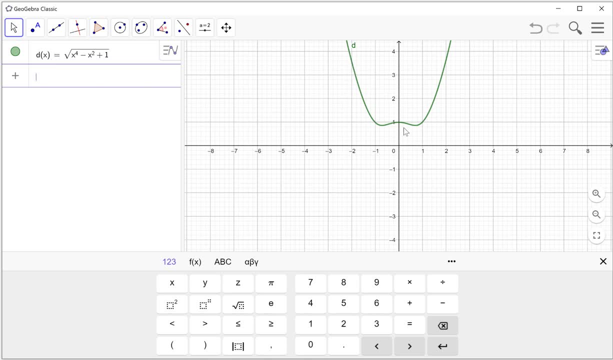 So notice that For negative, notice that as x gets bigger, so as x gets larger. this way the distance decreases, So our distance gets smaller and smaller and smaller to here. So somewhere in here is an x-coordinate where that distance bottoms out. 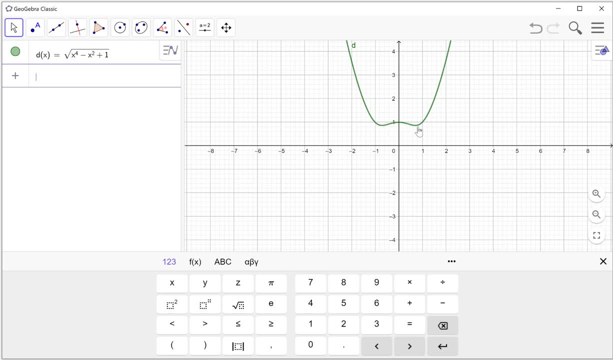 Then the distance increases for a while And then it bottoms out again over here And it looks like the function might be an even function. So it looks like we have some symmetry here. And then the distance, The distance increases as the x-coordinate gets bigger and bigger and bigger. 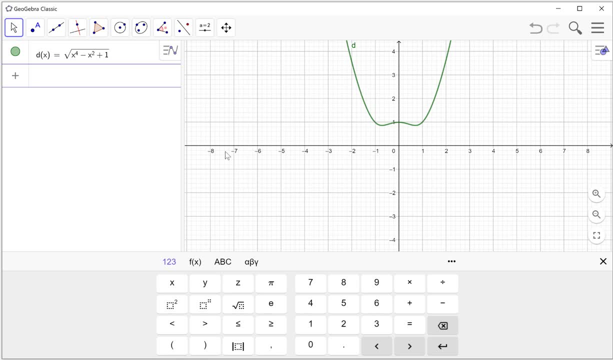 Now let's see if that makes sense with our picture. So, as x increased, the distance between the parabola and the origin got smaller until somewhere just past negative 1, increased again, decreased again and then got bigger. Well, let's see. 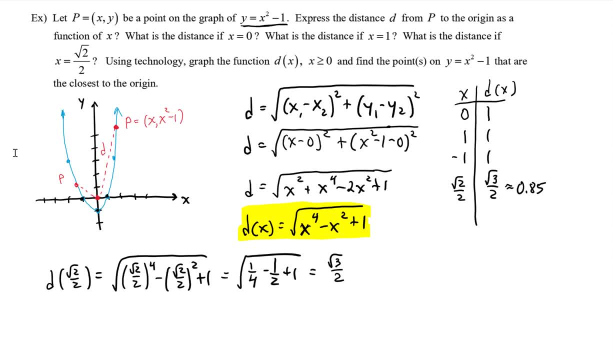 So my distance up here on the graph is pretty big. I'm pretty far away from the origin. As I come along the graph, though, my distance is shrinking, And then somewhere just past negative 1, so somewhere in here, apparently, I'm the closest. 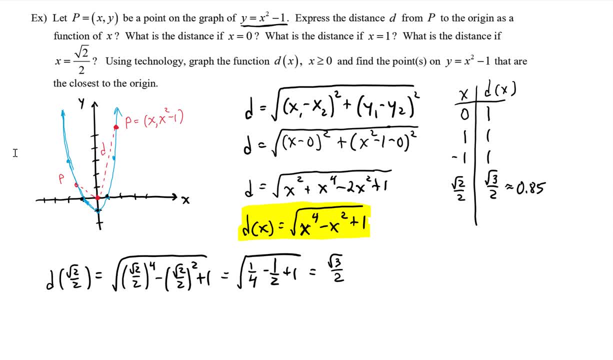 I'm ever going to be to the origin. Then I increase my distance to 1.. I go back through that- another point that's really, really super close, likely the closest to the origin- And then the distance increases. The distance from the origin increases the rest of the way. 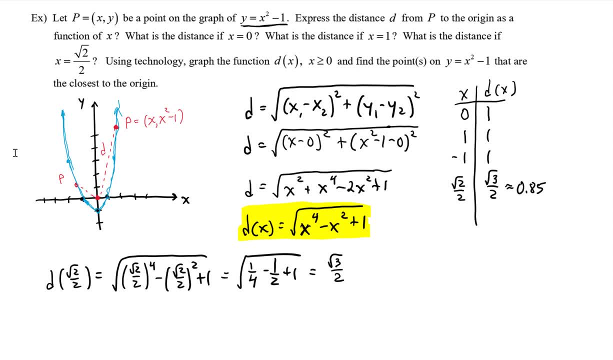 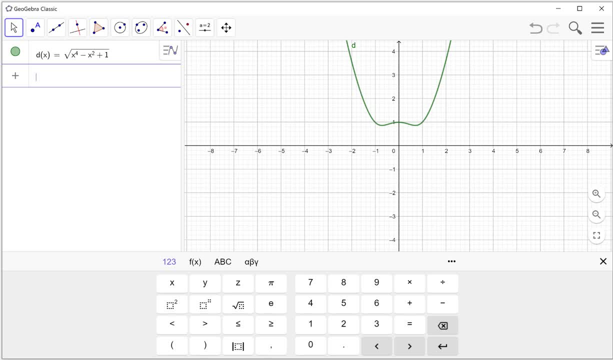 So that makes sense. My graph makes sense with what I'm seeing in this picture. Well, now we want to know what x coordinate do I need so that that distance is minimized. It's the smallest distance, So we can ask Geogebra for that. 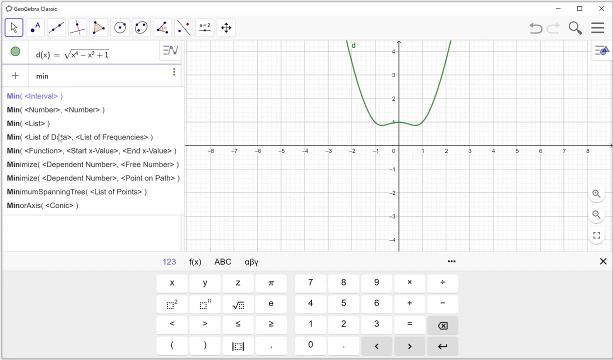 So we can type min and then we want this one, we want the minimum of a function, and then it's going to ask us for a starting x value and an ending x value. So our function was named d, so we can just use the name. 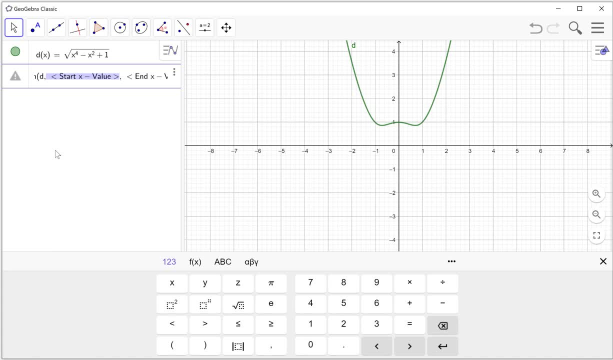 Our starting x value. So it did say to do positive x values. in our example, if you reread the example, it says: just consider positive x values, So let's start at 0. And my biggest x value. basically, where do I want to have Geogebra? stop looking for a. 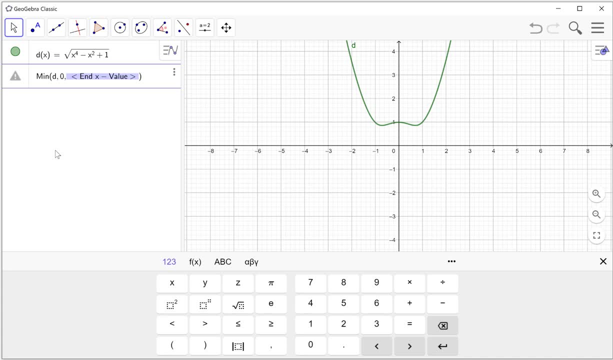 minimum value. I'd say it's. we don't need to look any further than x equals 2, because when x is 2, your distance is pretty big. It's way far away from this minimum distance. So let's have it go to 2, and we hit enter and sure enough it plots where we guessed. 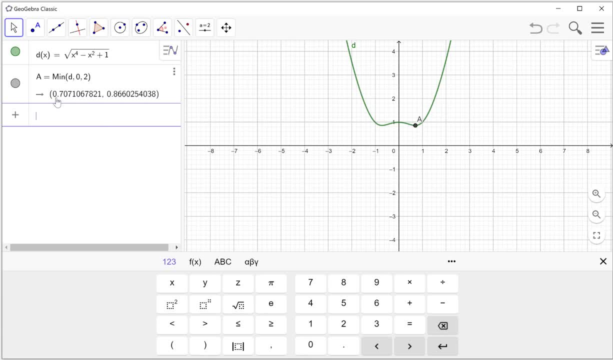 the smallest distance would be. and what is that x coordinate? That x coordinate is .7071067821, it's a decimal with quite a bit of accuracy. there we have quite a few decimal places. So we now have an x coordinate to work with that, we know, minimizes the distance between. 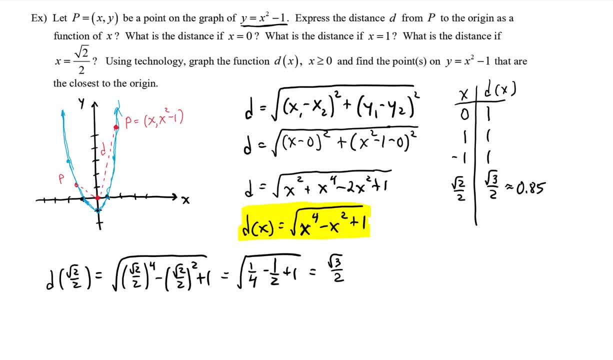 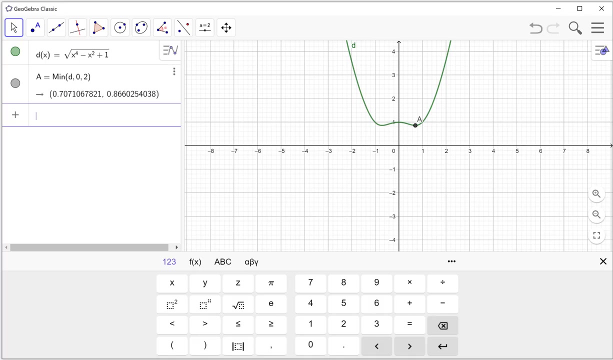 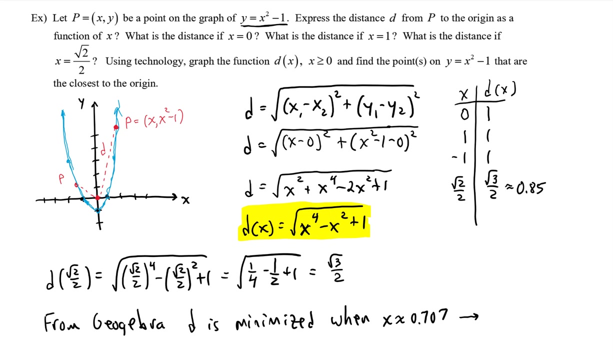 the parabola and the x And the origin. So from Geogebra, d is minimized when x is approximately .707.. But it turns out, and you can check this on your calculator, That's root 2 over 2, which is why I had you check that one. 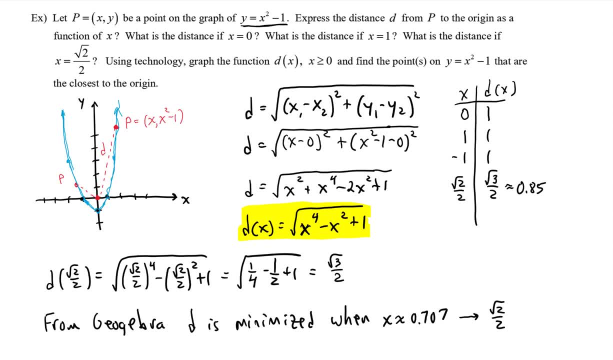 So it was at root 2 over 2.. Now we wouldn't necessarily know that if I didn't give you root 2 over 2 earlier, but you know, Geogebra would have given us a decimal that was really close to what we wanted and 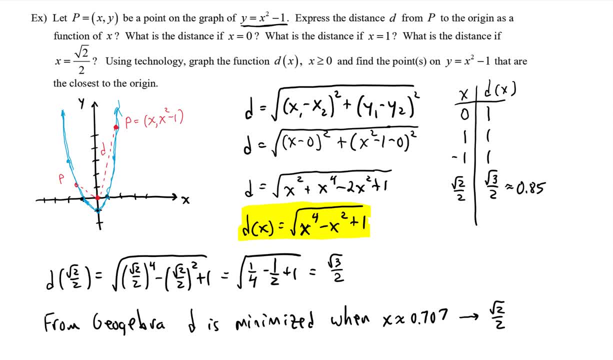 that would be good enough. We can get as much accuracy as we want using a computer, So we have a lot of decimal places of accuracy there. So it says: find the points on the parabola, On the parabola that are closest to the origin. 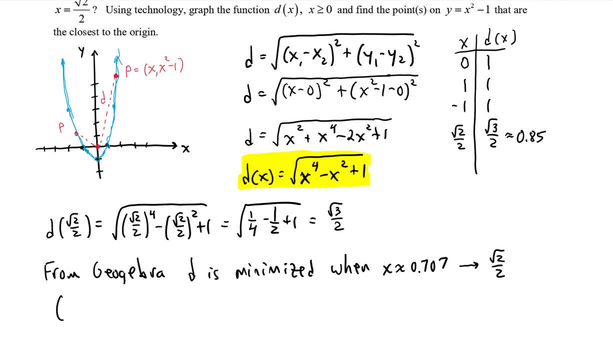 Well, now we can do that. So now it's going to be root 2 over 2,, negative root 2 over 2, because of the symmetry, right, You can go negative root 2 over 2,, unless we're just doing positive x values only. 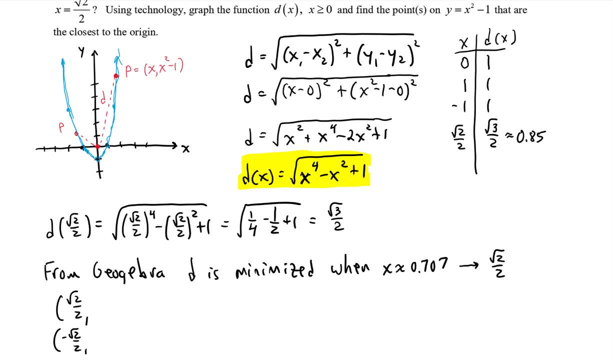 But it did want all the points on the parabola, so we'll go ahead and give both. So then we plug those in to the parabola. let's get the y coordinate. So y equals square root of 2 over 2.. 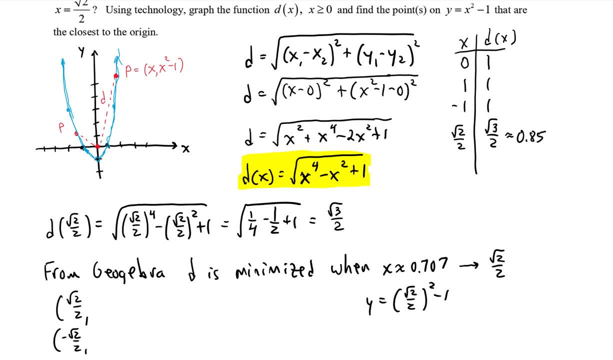 So we plug those in to the parabola to get the y coordinate. So y equals square root of 2 over 2.. So we plug those in to the parabola to get the y coordinate. So y equals square root of 2 over 2, squared minus 1.. 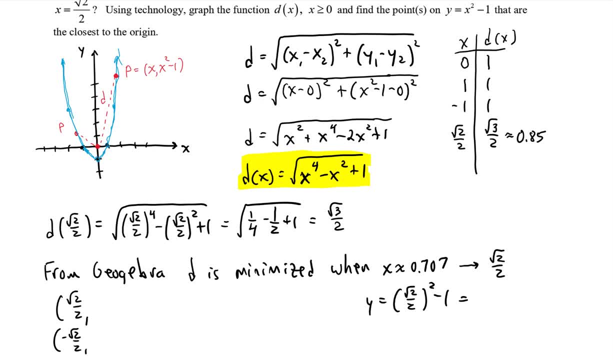 So that would be 2 fourths, which is 1 half minus 2 halves, be negative 1 half. So negative 1 half. So those coordinates right there, So basically right in here, is about as close as you're ever going to be to the origin. 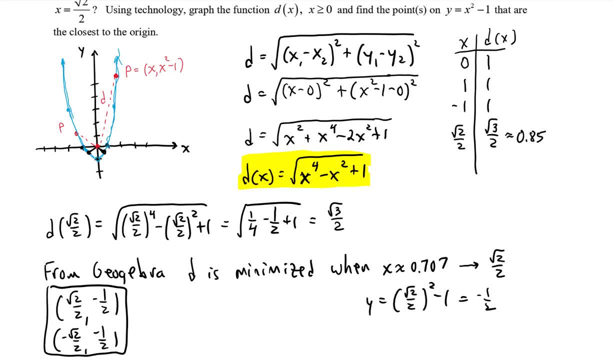 That's what we just found out. But again, the main thing We were practicing here is coming up with this function that models something we wanted it to model. So we came up with a function of x that when you plug in x, it gives you the distance between: 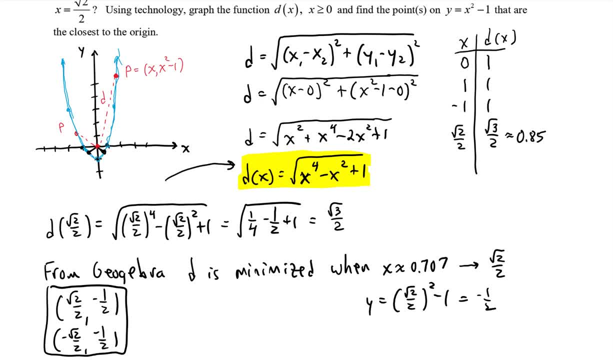 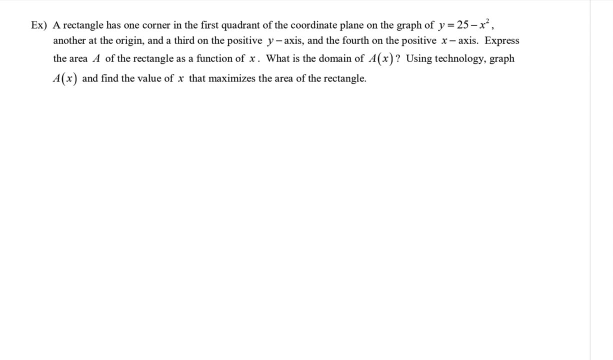 the point on the parabola and the origin. So that was the main idea here. The rest of this was just working with that function. Okay, let's take a look at another example. This time around, we're going to write a function that models area, specifically area of a rectangle. 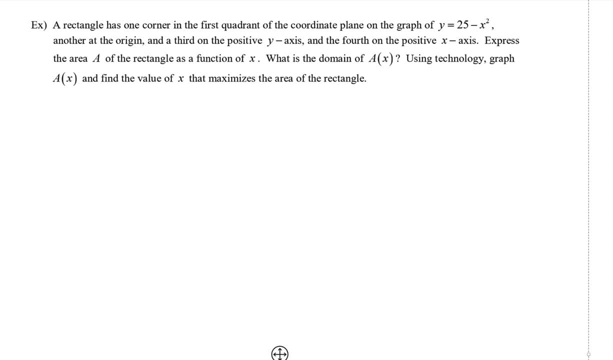 So a rectangle has one corner in the first quadrant of the coordinate plane on the graph of this parabola, another at the origin and a third on the positive y axis and the fourth on the positive x axis. Express the area of this rectangle as a function of x. 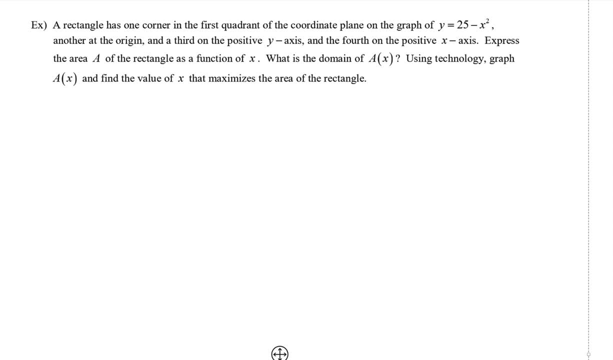 What's the domain? And then let's find the value of x that maximizes area. So we're going to model area this time instead of distance. So let's go ahead and draw a picture Again, I like to know what I'm looking at. 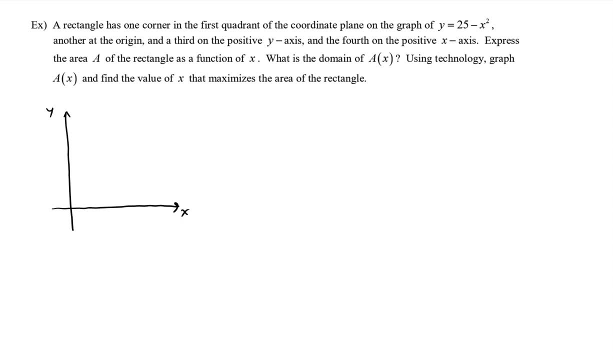 So we're just in the first quadrant. We've got the parabola 25 minus x squared, So that's the squaring function flipped upside down and shifted up 25.. So it's going to be up here at 25.. And then when x is 5, it's going to hit. I'm not going to draw this to scale, but when. 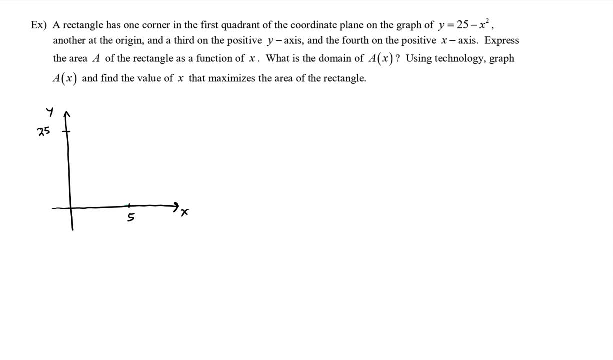 x is 5. It's going to hit the x axis. So basically it's this parabola here. Now we've got a rectangle that has a corner on this function, another one at the origin and then one on each axis. 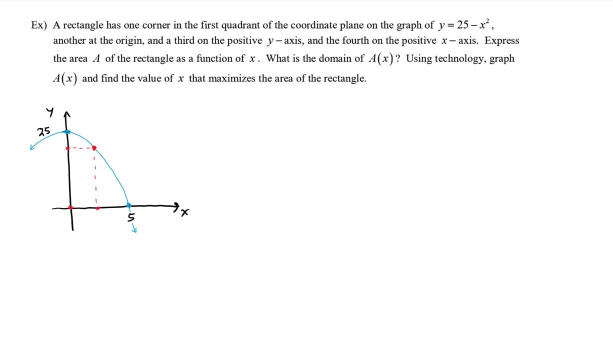 So this, for example, could be the rectangle, So that rectangle right there Now this point would be x comma, 25 minus x squared, Where this is the distance x And then this is the distance 25 minus x squared. We go right x and up 25 minus x squared. 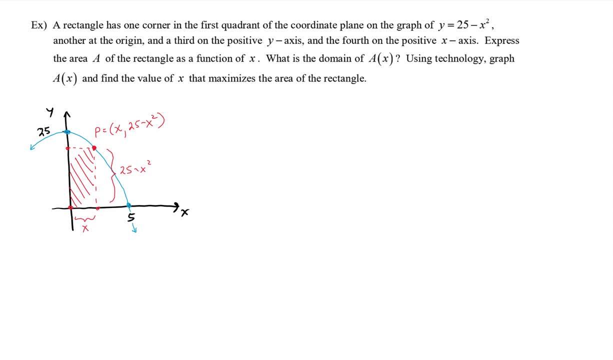 Now, depending on where that point is, you'd get a bigger or smaller rectangle with different areas. So if the point was way over here, then your rectangle would look like this, which would have a different area. So we're trying to find where you'd have the point. 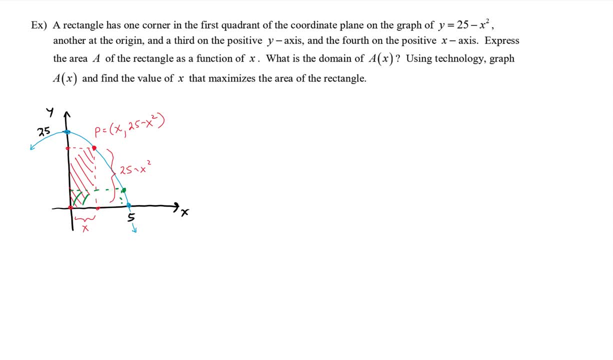 Okay, So we'd have the biggest area, Most area. We want to maximize area, So let's see if we can do that. So area of any rectangle is length times width. So area for us as a function of x would be x times 25 minus x squared. 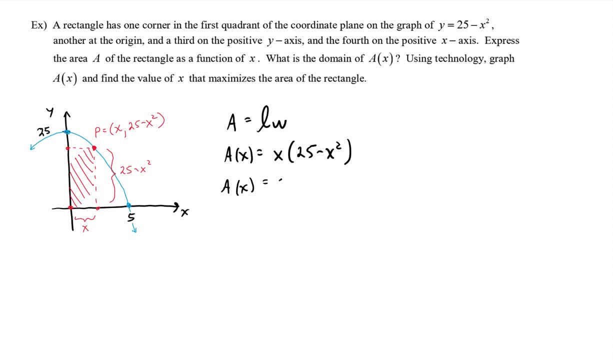 If we want to multiply that out- Which we don't really have to, but if we wanted to, it would be 25x minus x, cubed. Now it says that x has to be on the parabola and in the first quadrant. 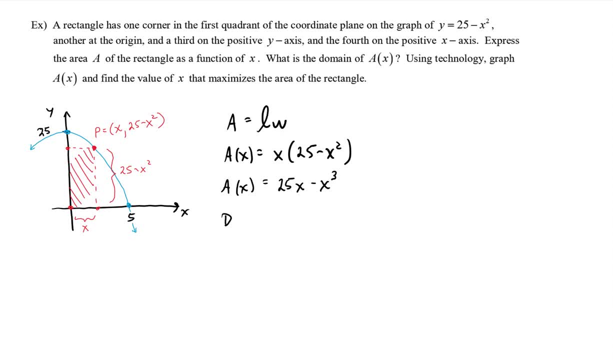 So there is an implied domain here, The domain to be in the first quadrant and on the parabola You can't be smaller than zero and you can't be bigger than five. If we went past five it wouldn't be in the first quadrant. 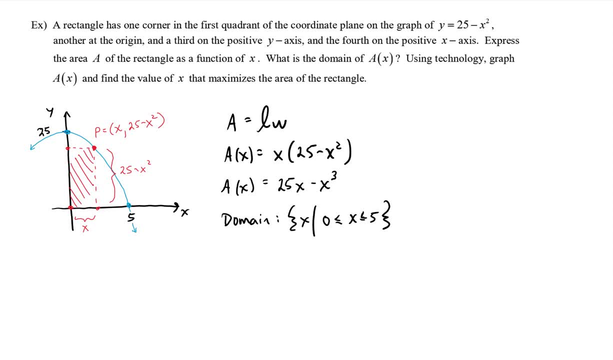 So we only care about x values from zero to five. Now we're trying to find the value of x. that would give us a rectangle with the most area. So again, we could guess and check by plugging in x values. but at this point we really just 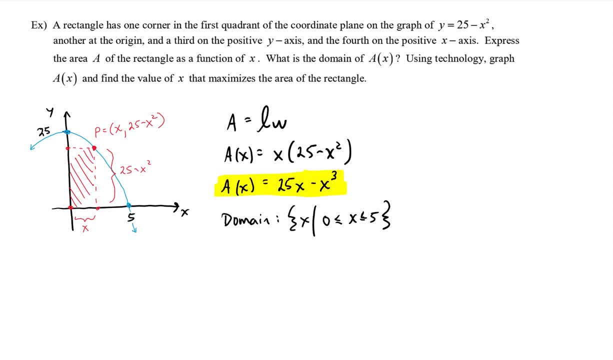 want to model coming up with this function, which is what we just did. So that's kind of the main idea here. This was our big moment, And then we're just going to use technology To actually go find that value of x. 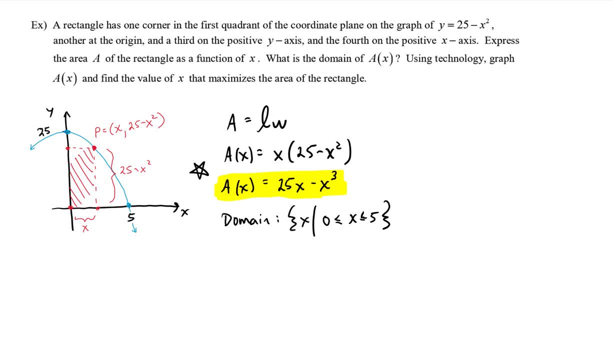 So as you progress through mathematics you learn lots of different ways to maximize or minimize a function. Calculus shows you how to do that in a lot of cases without using technology. But we're just going to use technology to find the value of x that maximizes that area. 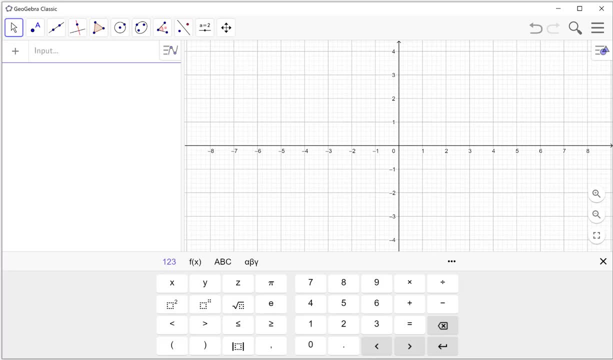 Okay, so we called our function x And we had 25x minus x to the third. I believe 25x minus x to the third. yes, So when we graph that, we can't see all of it, So we're going to want to zoom out. 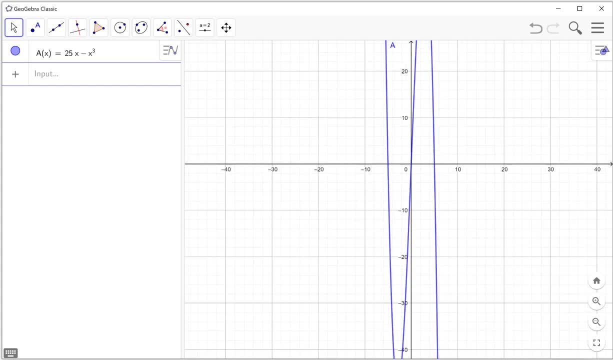 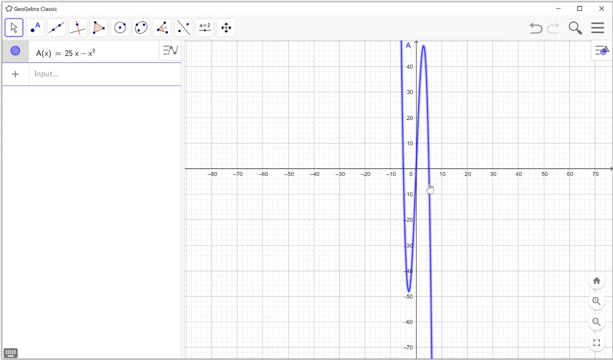 And again, we only care about x being zero to five. So if we zoom way out We can see that here's zero, And before we get to 10, there is a maximum value of a. There is a point at which a goes no higher. 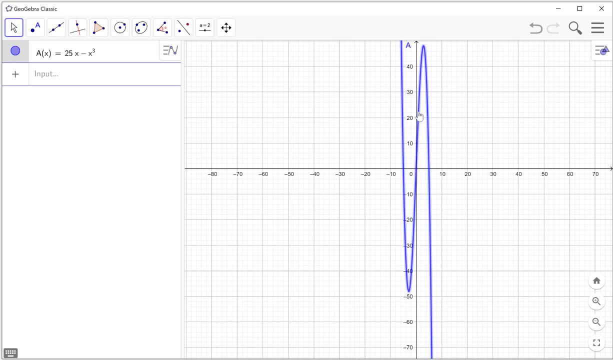 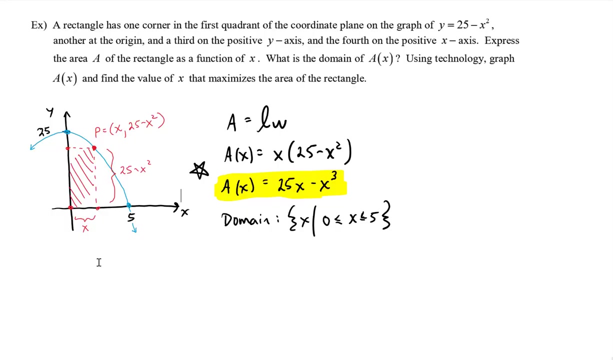 So as x gets bigger from zero, the area of the rectangle increases And the area reaches its maximum value here, And then the area starts to get smaller as the x coordinate gets bigger and bigger, closer to five. So I think we'd agree that if your x coordinate was five, if you were way over here then 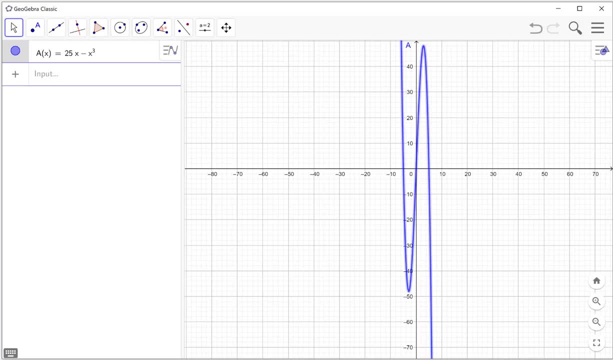 there'd be no height to your rectangle, so the area would be zero. So when we look at this area function, when x is zero, the area is zero And then, as your x coordinate gets bigger, the area inside your rectangle gets bigger. 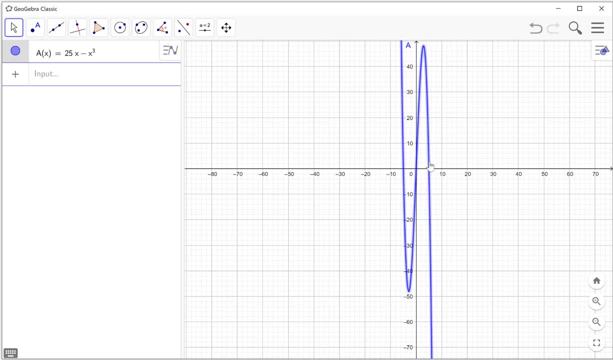 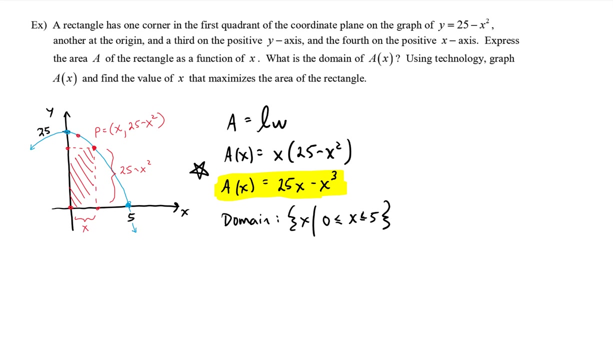 Until you get to here, though. then the area starts to get smaller as the x coordinate takes its way over to five. So when you're up here and you're working your way over, your area is getting larger and larger and larger. 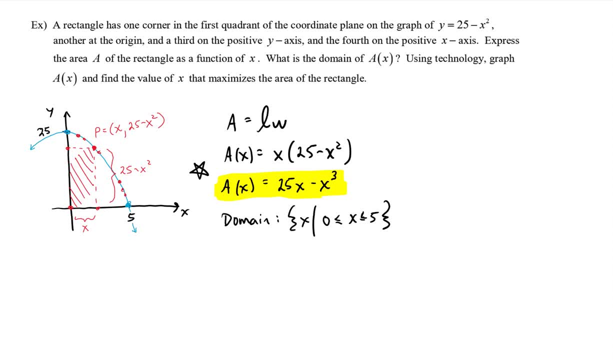 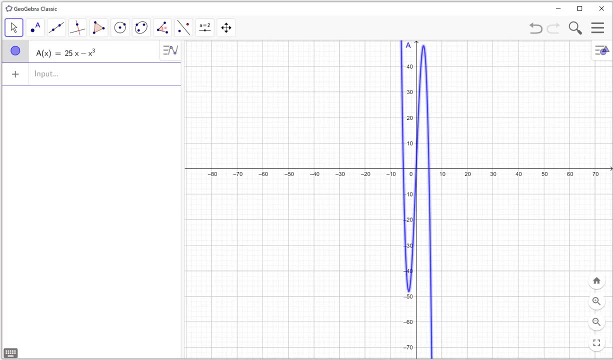 But there comes a time where, when you start to get close to five, the triangle starts to get less and less area. So we just need to figure out where that occurs. So, again, we can just ask GeoGebra to do this for us. 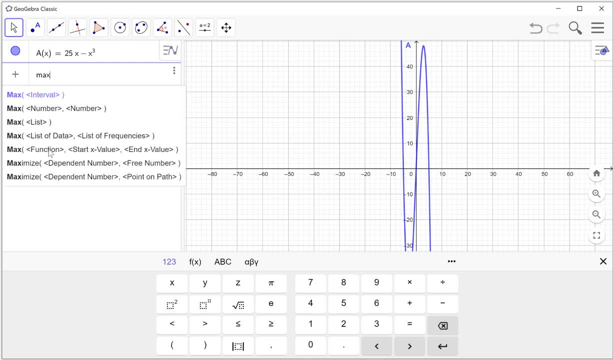 We're just going to ask for the max of function, a starting at zero going to five, And it plots it for us and tells us that that x coordinate is 2.8867513,. we've got a whole lot of decimal places we could work with here, but we'll just do 2.89,. let's go. 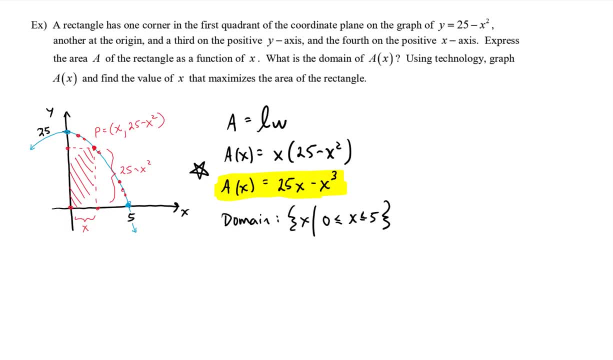 ahead and round 2.89.. So from GeoGebra, Okay, The function a is maximized when x is approximately 2.89, so let's go with that. it's good enough. We could get more decimal places if we wanted to from GeoGebra, but that should work just. 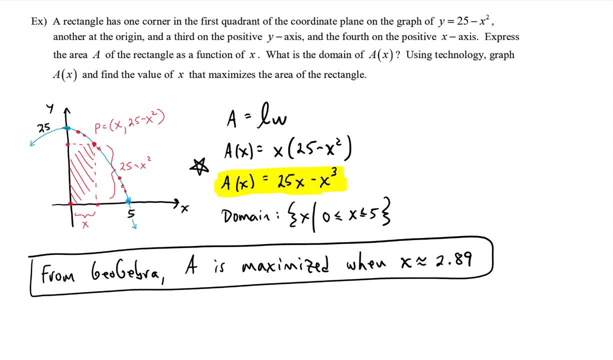 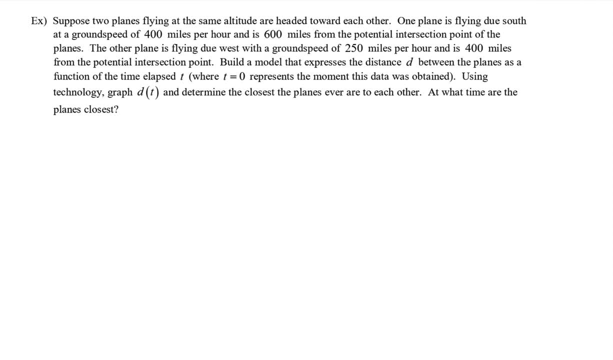 fine. Okay, Let's take a look at one more. In this last one, we've got two planes that are at the same altitude headed towards each other. One's flying due south and the other one's flying due west, and we know the rate at which. 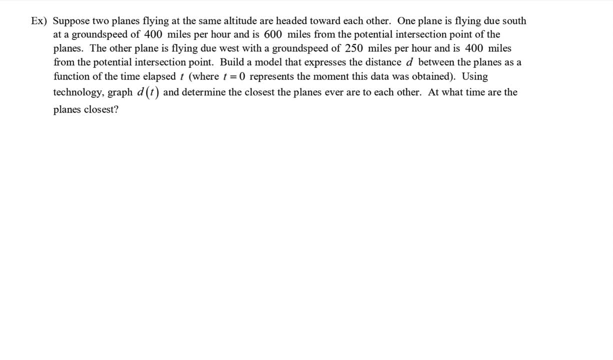 they're moving through the air. we actually know the ground speeds. we're not going to worry about whether there's a headwind or a tailwind and pushing them faster or slowing them down. we're just going to take all that out of it. at least know how fast they'd be. 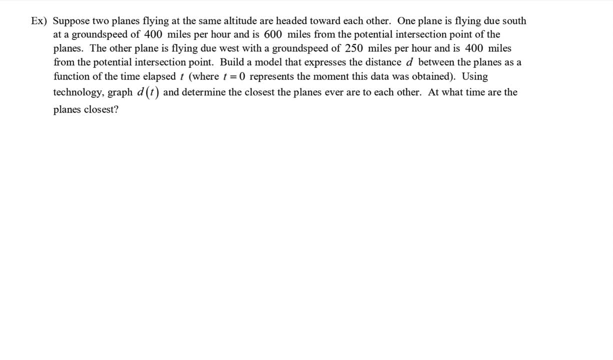 going on the ground And we're interested in knowing how close these planes will come to each other. so they're not going to hit each other. so how close do they actually come? let's see if we can't figure that out. So we're going to model distance again. 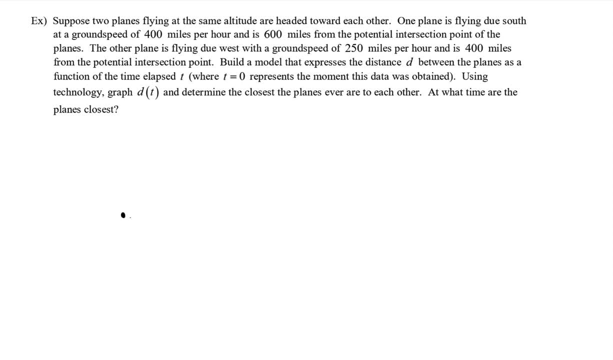 So let's say: this is the possible point of impact. Okay, So, this is the possible point of impact, Okay. Okay, So we've got two planes. of course I'm not going to have them hit each other. it's a. 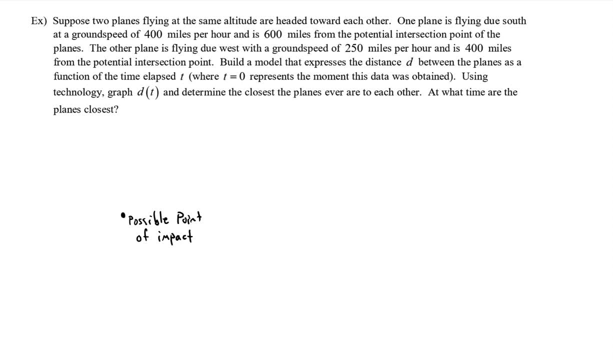 little morbid, so let's just see how close they come to each other. So we've got one plane that's flying due south, so it's headed this way. We've got another plane headed due west, so here's a plane, let's call that plane one. 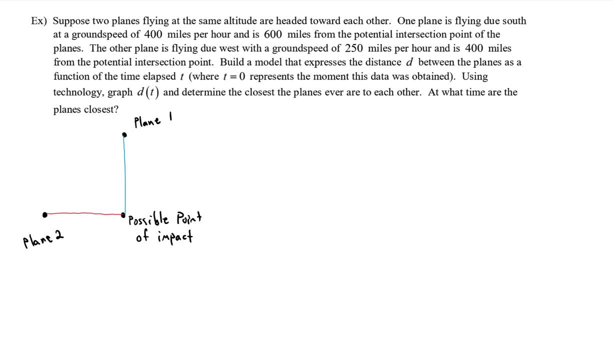 here's a plane- Okay, Let's call that plane two- And we want to know the distance between them. so we want to know this distance right here. Call that d, And we want to know what the minimum value of d is. if d is zero, that means they're going. 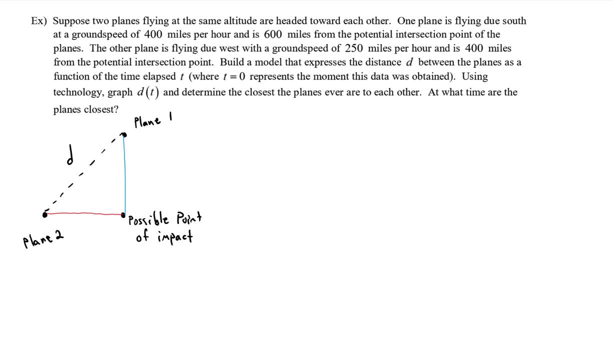 to hit each other. but I'm not going to give you one where the two planes hit each other. So we just want to see what the minimum value of d is in this situation. Well, the distance from this point to this point, We know how fast plane one- the one going due south- is traveling. the one going due 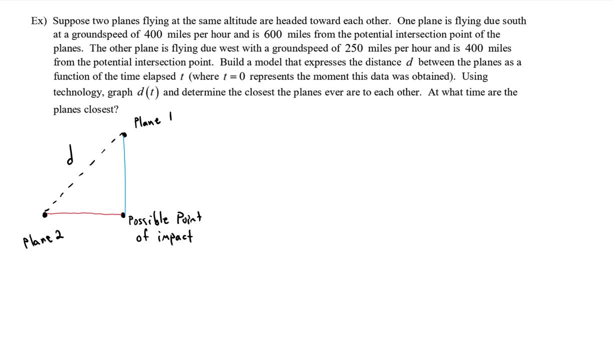 south is 400 miles every hour. So we know the distance equals rate times time. So this one's going 400 miles an hour every hour, where t is in hours, Okay, Okay, Okay, Okay. And the one going due west is going 600 miles per hour every hour. 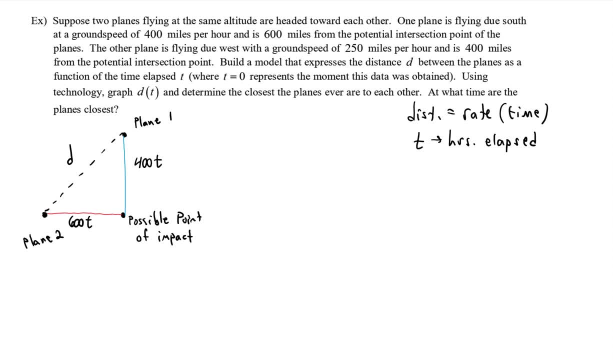 So at any time if I want to know how far apart this plane is from here. well, we got to be a little careful, though, because t equals zero represents the moment the data was obtained. It would help if I don't know. Okay. 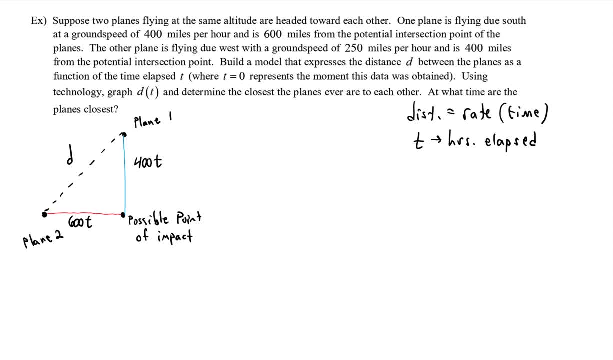 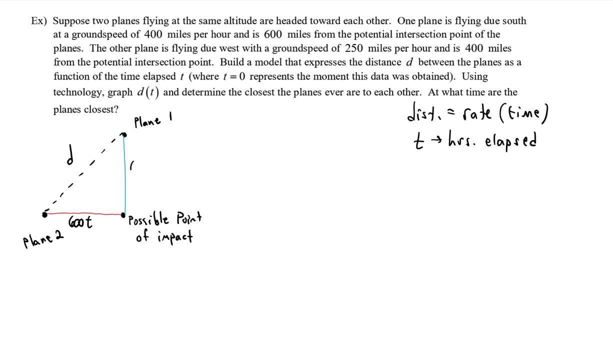 So this distance is 600, and then the other one is going ground speed at 250 and is 400 miles from the point of intersection, So this is 400.. However, Okay, planes are flying towards this possible point of impact. So, as time goes on, this 600 miles. 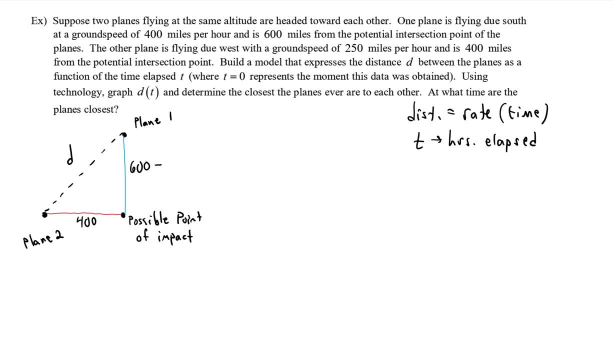 is shrinking by 400 t miles because that's how fast the plane is going. So if I take the 400 miles an hour, that plane 1 is traveling times how many hours it's gone. that's the distance it's covered from here to here. 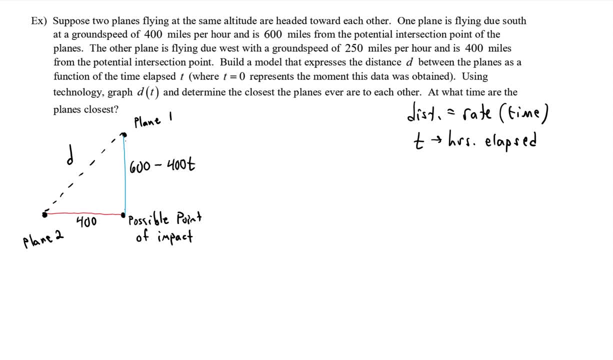 But it started 600 miles away. So, for example, if t was 0, then it's 600 miles away, But one hour later it's gone 400 miles. So 600 minus 400 would be 200. This is 200 miles. 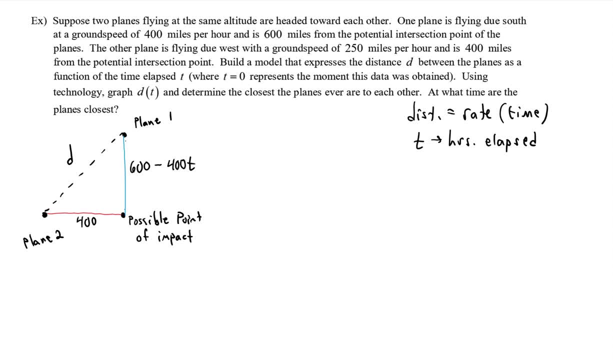 And then over here on this side in a similar fashion. we'd start with the 400, but then we're going to lose 250 miles every hour. Again, if t was 0,, they're 400 miles apart. If t was 1,, they'd be 150 miles apart. 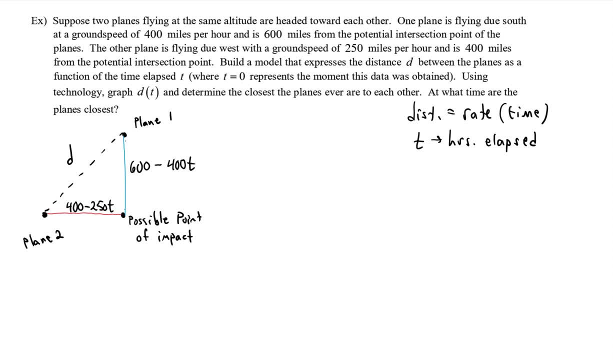 because in one hour it's traveled 250 miles. So now d is just part of a right triangle. So d squared would be the leg squared plus the other leg squared, Then d itself. I could square root both sides. However, d is a distance. 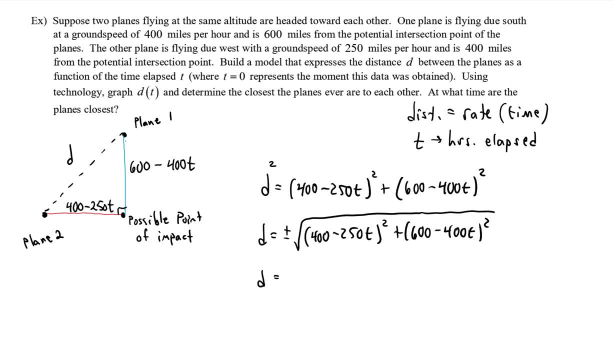 I'm only interested in the positive solution to this equation. So 1 times d squared times 1 times 1 minus alpha Tit of t squared 장님. So once again we have built a function that models the distance between these two planes. 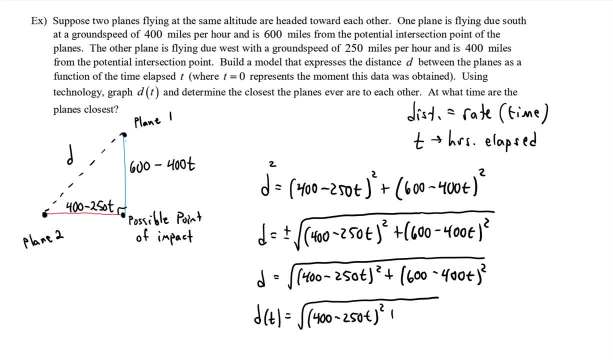 which is the main idea: d squared 2 times 1 x, t squared, You mightrant thing. we're practicing here how to come up with this and then again using technology, let's graph that and see if we can't figure out the closest the. 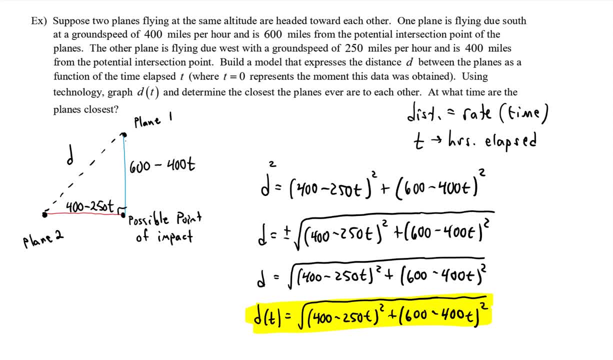 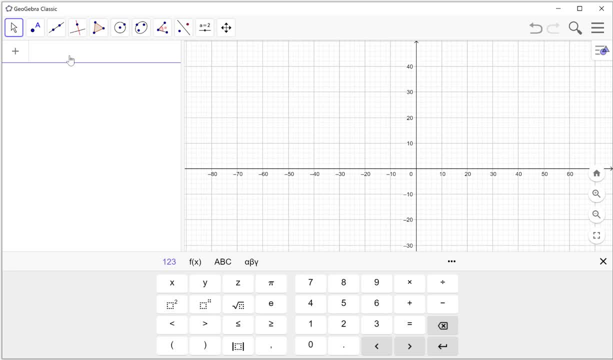 planes ever are to each other. so let's see if we can't get that distance real quick using GeoGebra. so we have 400 minus 250 X squared plus 600 minus 400 X squared. let's check right. so we've graphed that, but we can't see it. the numbers are rather large to zoom. 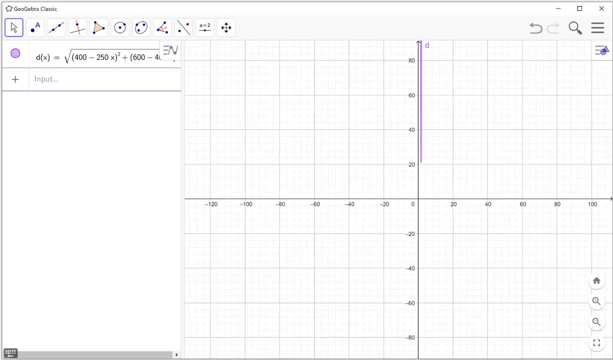 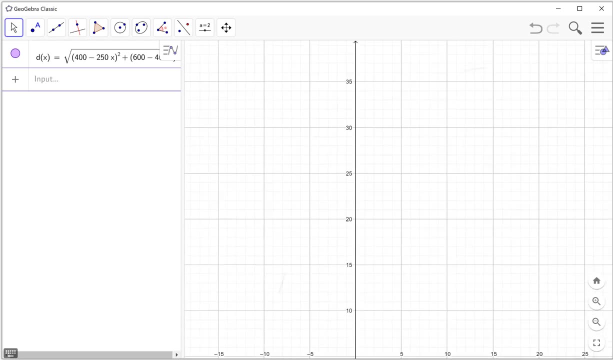 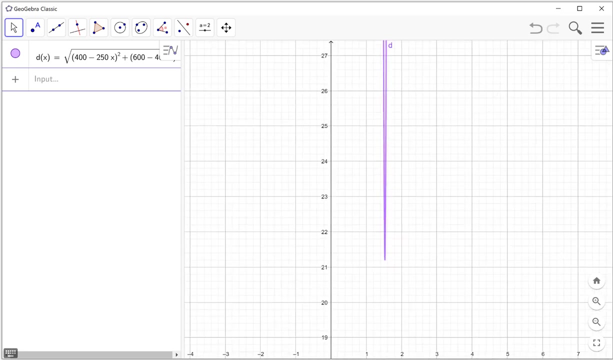 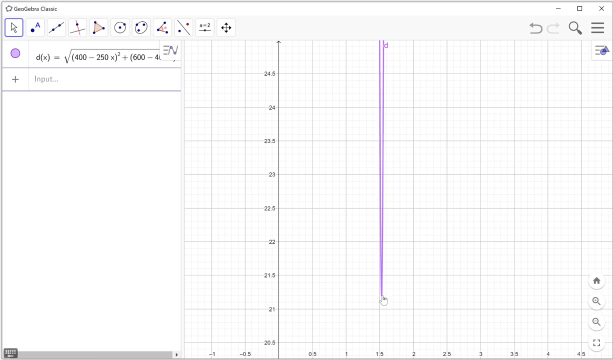 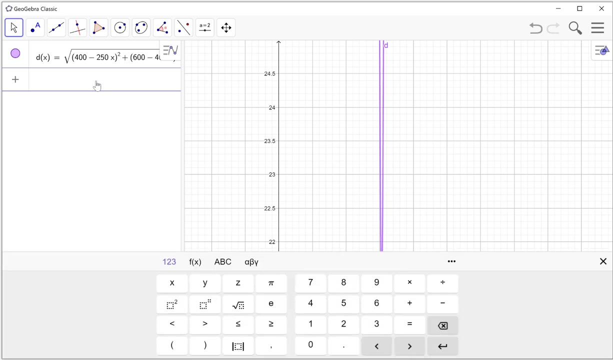 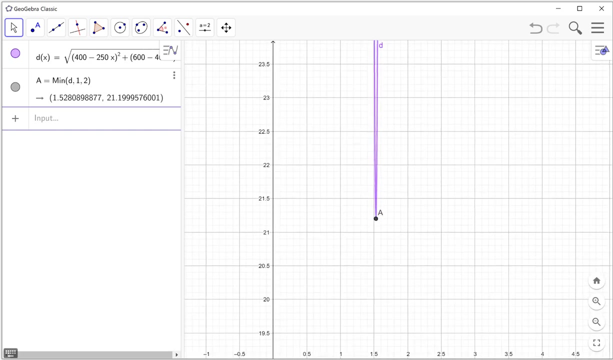 out. so let's see, it's hard to see zoom in, but we, if you look carefully, we can't see D decreasing to a point and then increasing. so there's that, that minimum distance that we're looking for. so let's do the min of D between 1 and 2, and there's that point. 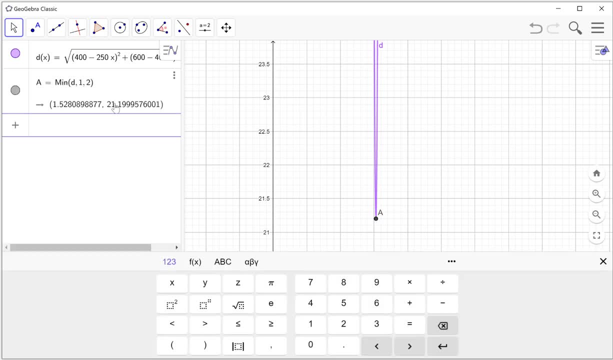 right there, and that minimum distance 21.199. oh, let's call that 20 plus g, so the normal stuff is the way to get 21.199. and let's do 86 and 96 on thekem return on that, so constant, probably cooked up and sharp, thatCam dot we're, and that minimum distance is 21.199, so let's call that 21.199. so let's go 20.199. 1 and i guess at 3 or 7 and 3 is en eladin, so at least 4.. communications of on thekem A2, behind by C or D vraag Straßenfurt in Bergen, Berlin and Germany".